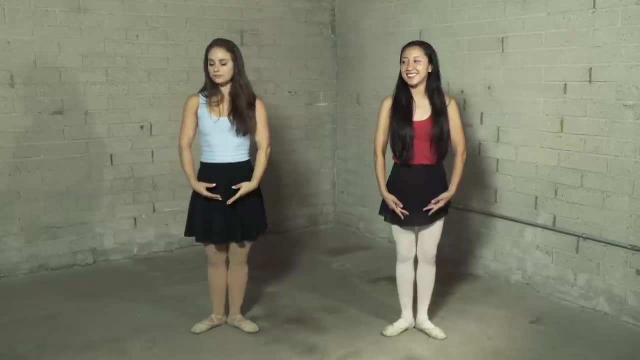 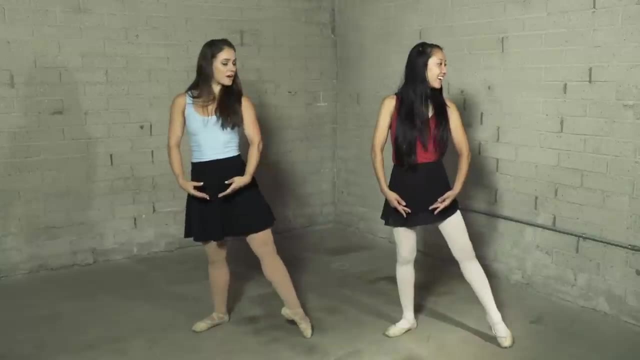 Can we do it together? Let's try four times. Here we go: One And in, And two And in, Three And in Last one, Four And back in Nice job. Give someone a high five, Yes. 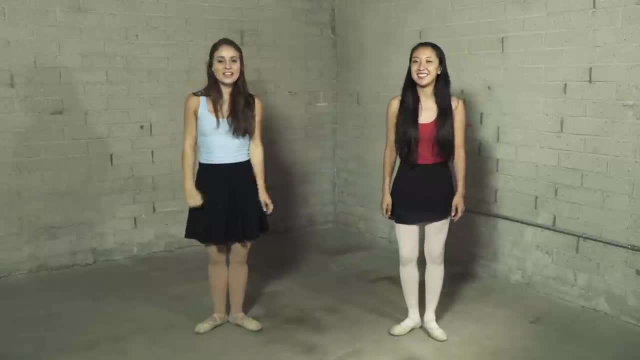 That was awesome. Or yourself, Give yourself a high five, Shake your legs out. So you guys did the first move. Can we learn the second one? Let's do it, Let's do it. So the second move is a plie. 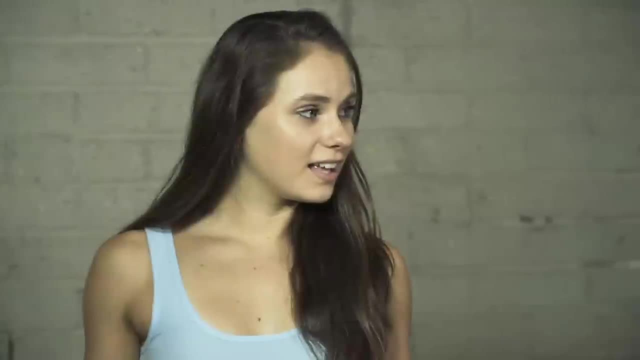 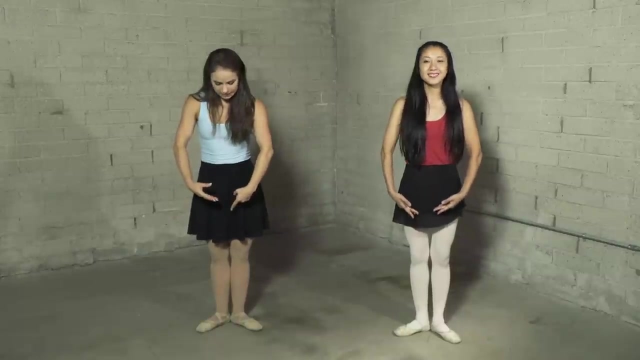 Do you guys know what a plie is? I think plie means to bend. It does mean to bend And we're going to be bending our legs. So go back to grabbing those flowers. Your heels are kissed nice and tight together. 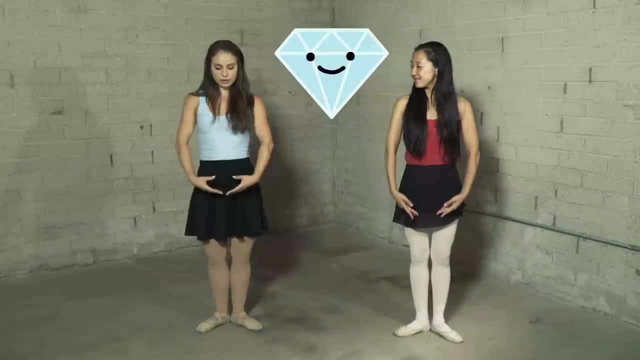 From here you're going to make a diamond shape with your legs. So your knees open wide. You sink down just a little bit And then straighten those legs. Okay, Let's do it again. Let's do it again. Let's do it again. 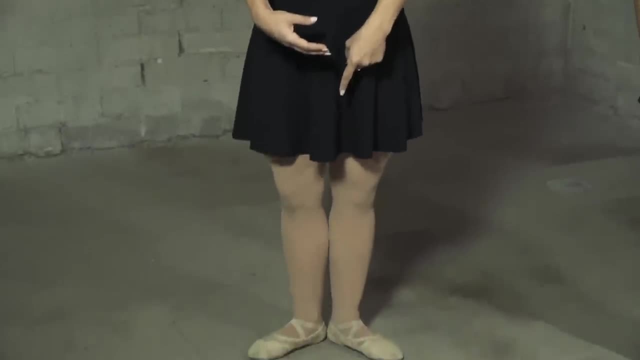 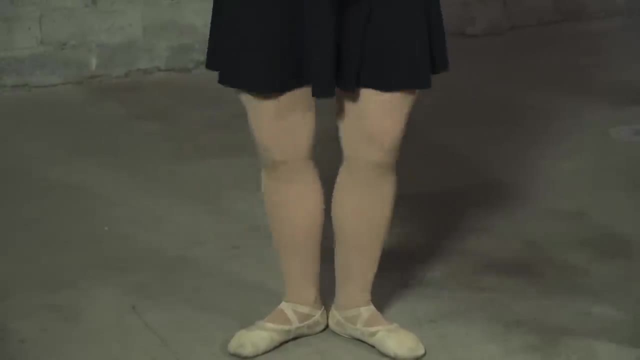 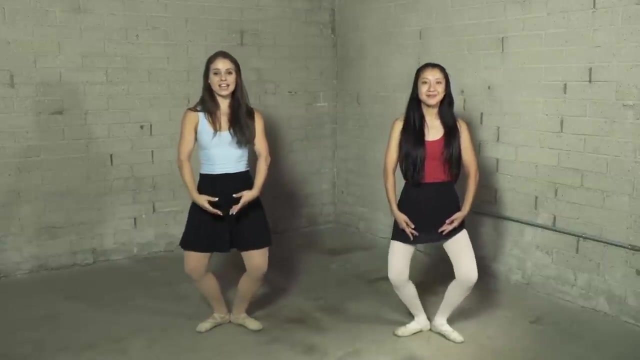 You want to keep your heels glued tight to the ground, And then you straighten up. Here we go: Plie And straight. Again Plie And straight. Two more Plie And straight. Last one Plie. 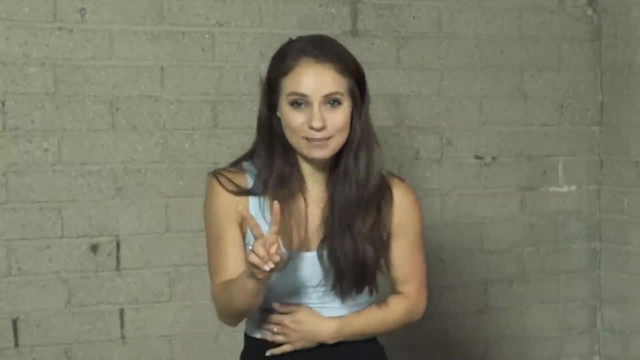 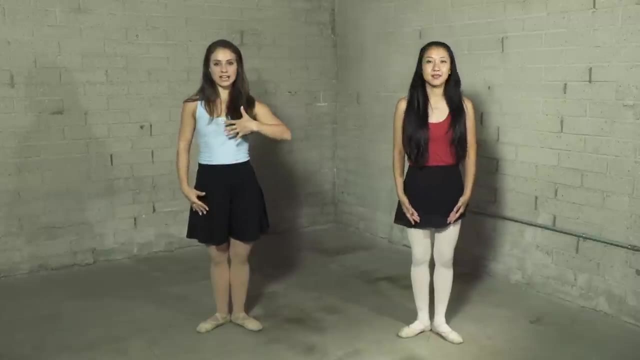 And straight. Nice job. You guys learned your second move. Are you ready for the third one? Okay, This one's kind of tricky, So put on your brave face. You guys got it. You got this From here from your first position. 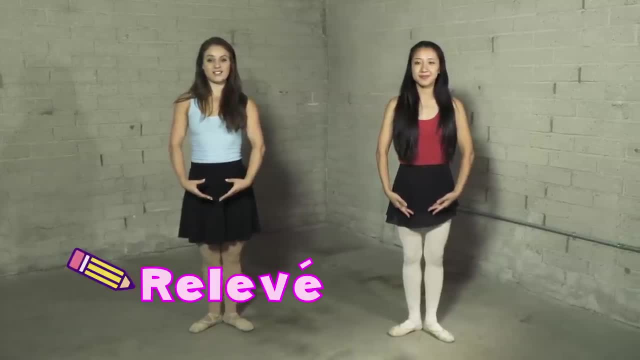 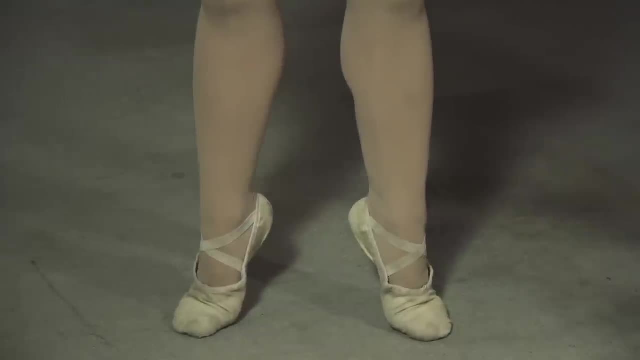 your arms holding your flowers. all you're going to do is releve. That means to rise up on your toes- Perfect, Nice and tight. Pull your abs in your belly- nice and strong- And then take your heels back down to the ground. 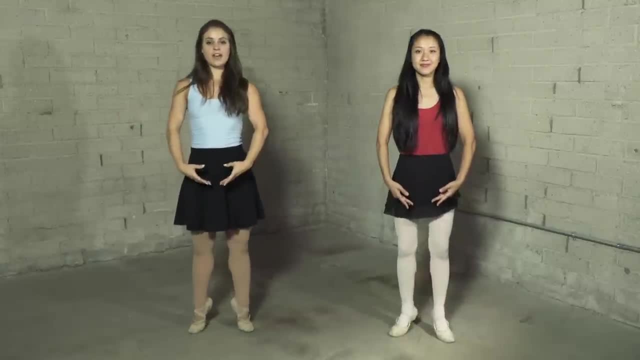 That's all there is to it. Let's try a couple more. Let's go up, releve And back down. Good Up, releve And back down. Last one: Up and hold it, Hold it, hold it as long as you can. 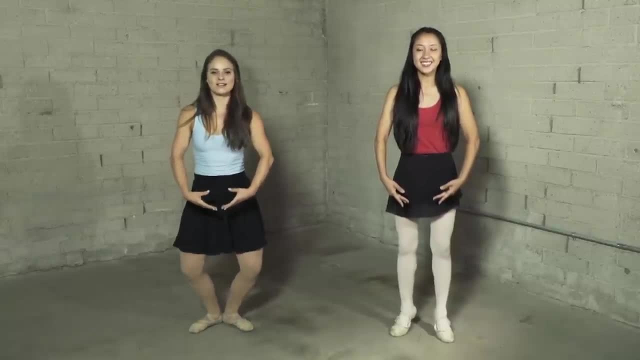 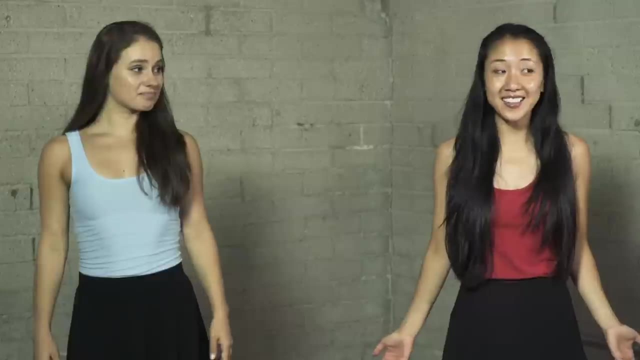 Try not to wobble, but it's okay if you fall And come back down to your toes. Awesome job, you guys. How do you feel Good? I feel pretty good. I think we can do one more move, You think so? 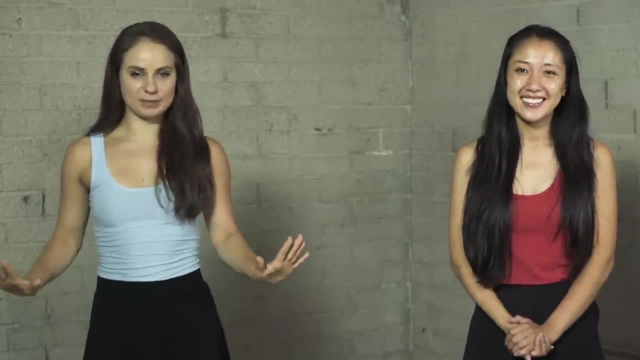 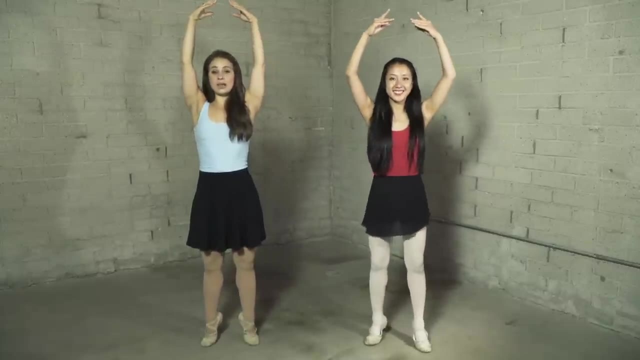 Let's do a bonus one. You guys ready too? Okay, So this is our bonus move. It's called a bourree turn. All you're going to do is stand up to releve on your tippy toes and pull your bellies in. 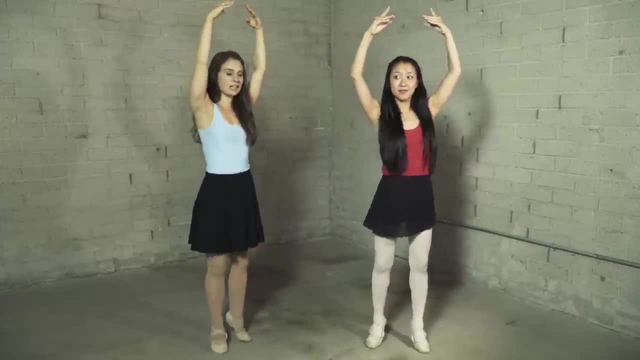 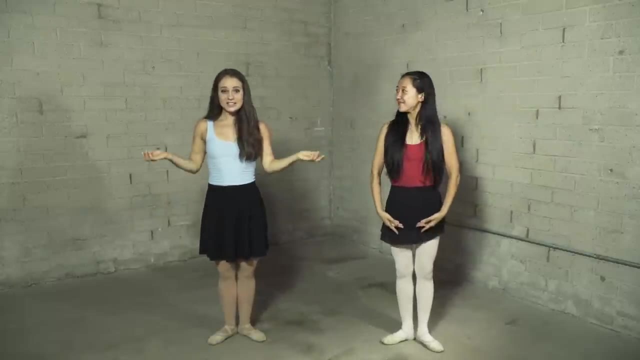 nice and tight, because you're going to do tiny little steps with your feet and turn around in a big circle and come back to the front and go back down to your first position. That's all it is. Let's try it a couple more times. 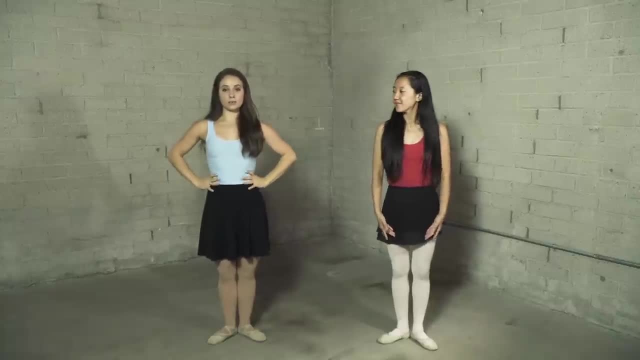 And if you need some help balancing, just grab onto your waist, Put your hands down here. I'll keep my hands here and if you're ready to put your arms up above your head, you can watch Nua. Ready Up on your toes and releve. 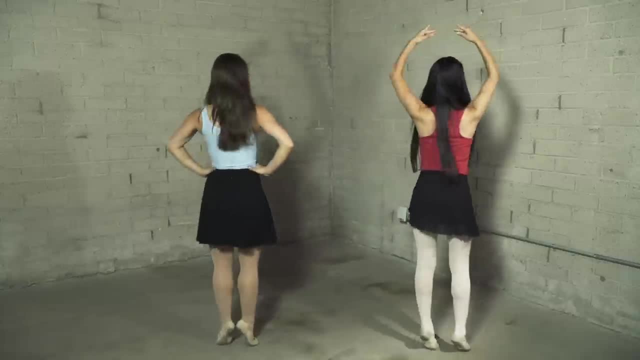 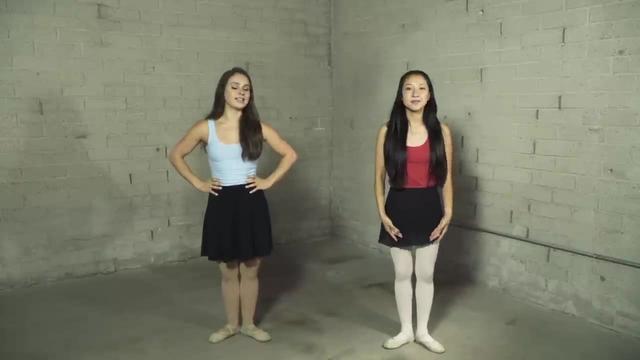 And tiny little tiptoe steps all around like you're sneaking to see your presents on Christmas morning and come back down. Nice guys, Let's try one more. We're all together and then we'll put it at the end of our combination. 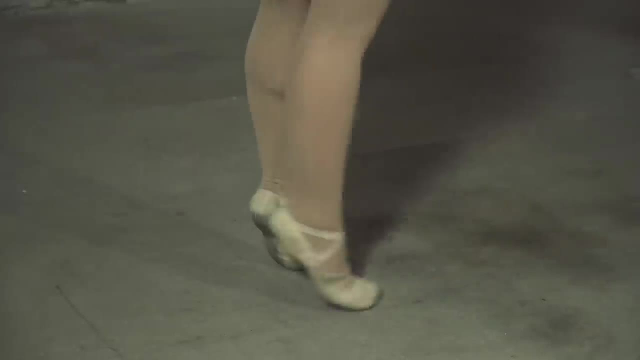 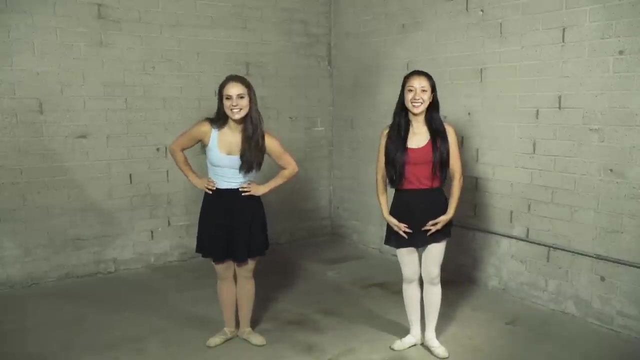 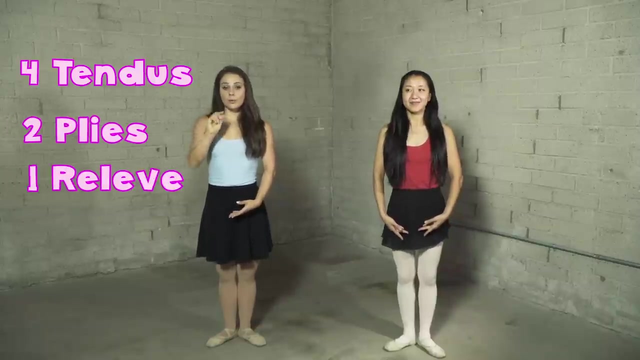 Up on your toes, tiny little steps all the way around in a circle and back down. Wow, That was awesome. You did great. Let's try it together. So, from first position: four tendus, two plies, one releve and spin it around, and then we'll. 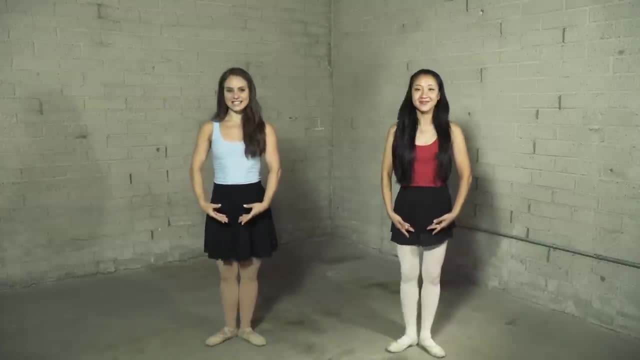 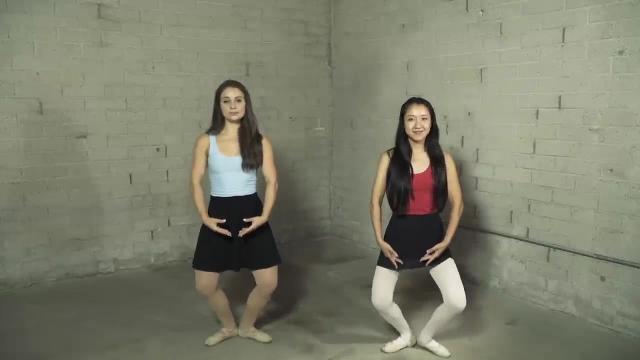 finish, Here we go. Tendu Together, Tendu Together. Last one Plie, Here we go. Plie All the way up on your toes and bourree, bourree, bourree, bourree, bourree. 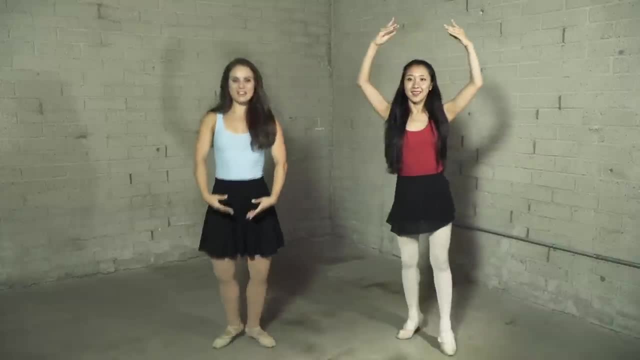 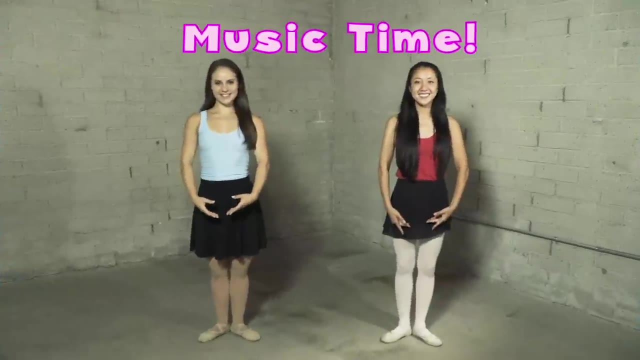 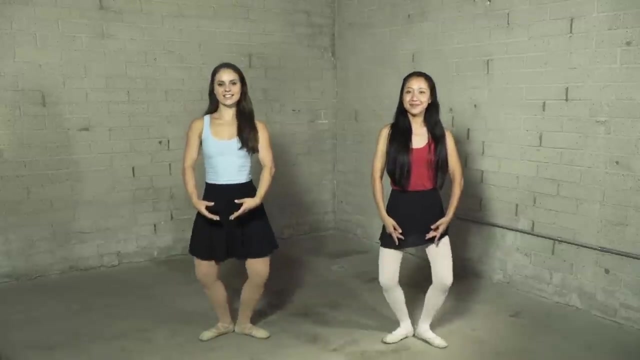 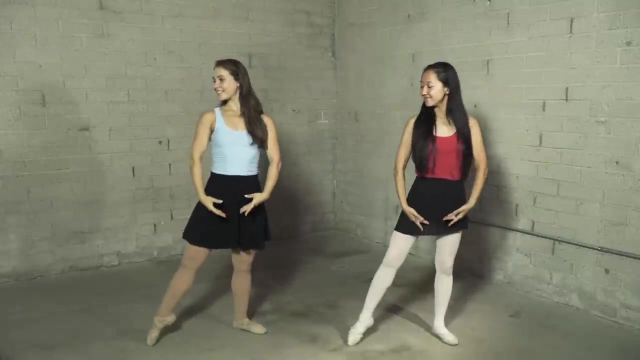 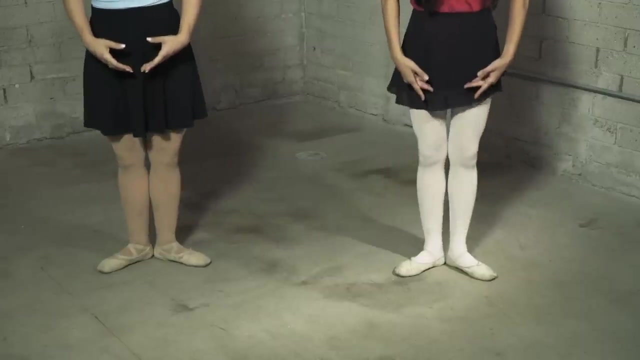 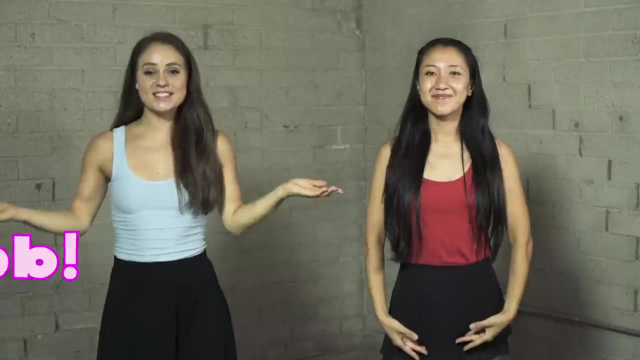 And flat. Nice job, guys. Let's try it again with the music and have a little fun with it. Great job, you guys, And don't forget to keep practicing at home. We'll see you guys, next time. Bye, Bye. 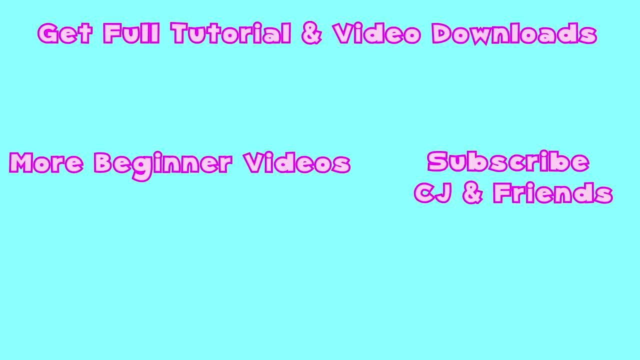